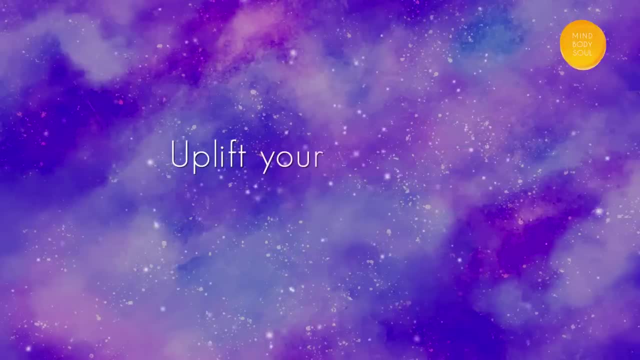 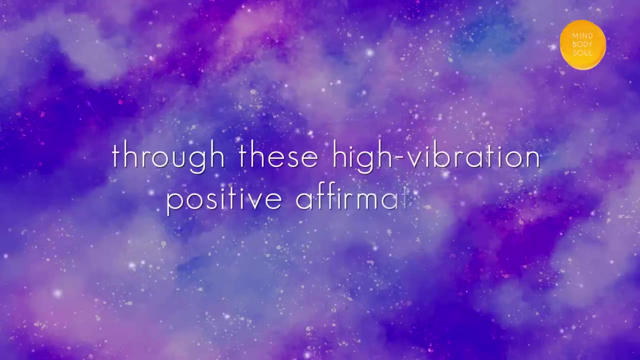 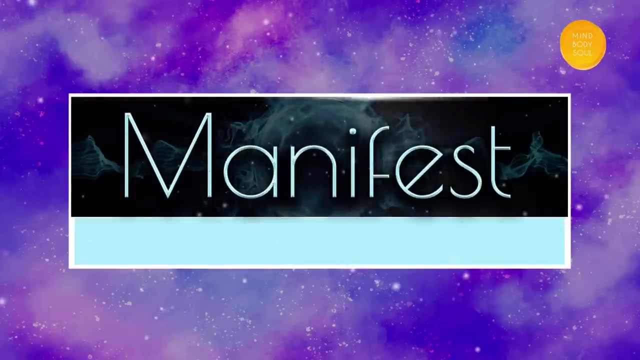 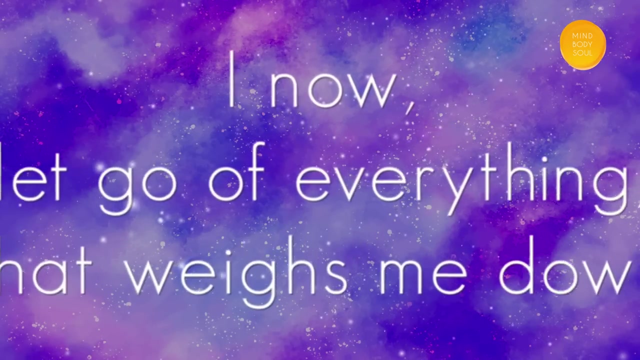 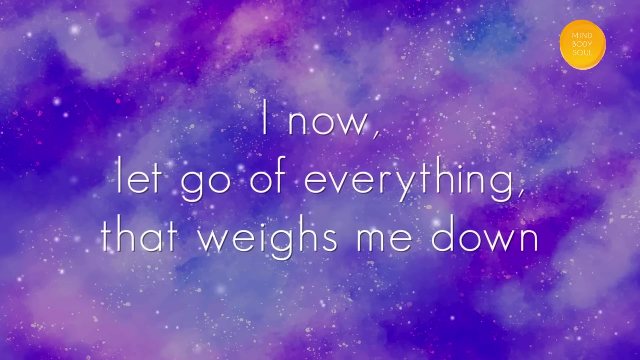 Words have the power to uplift. Uplift your vibration and let go of all the negativity through these high vibration, positive affirmations. Let's begin. I now let go of everything that weighs me down. I now let go of everything that weighs me down. 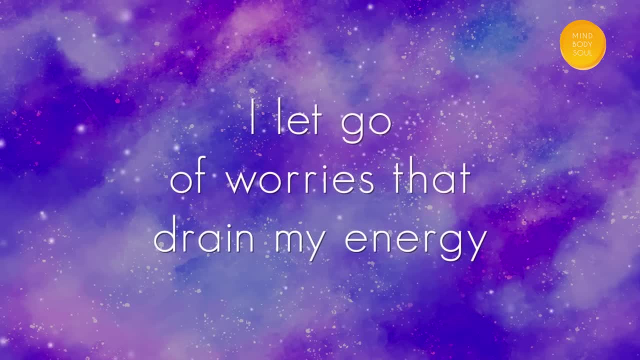 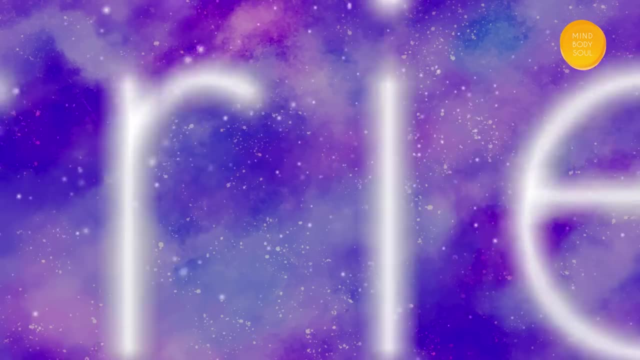 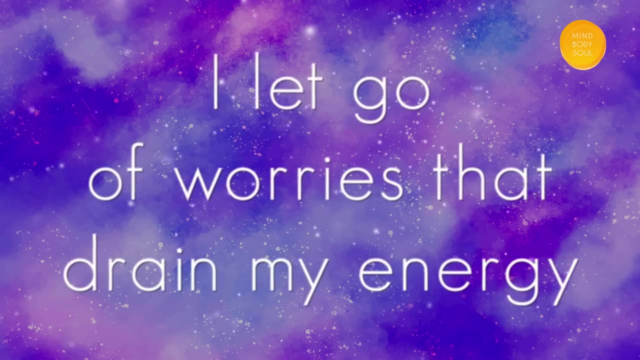 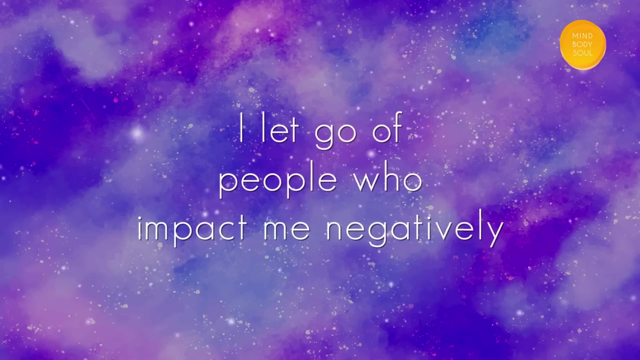 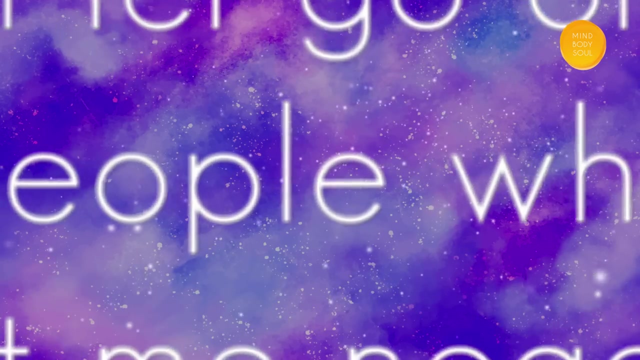 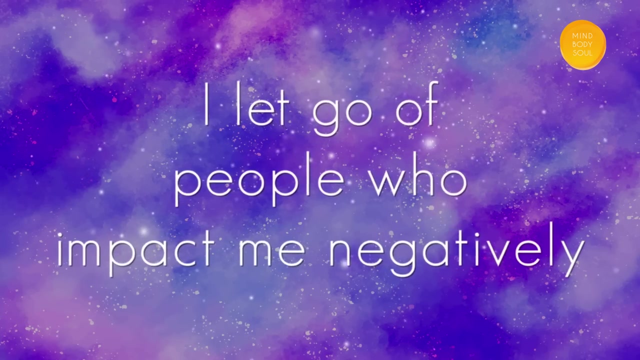 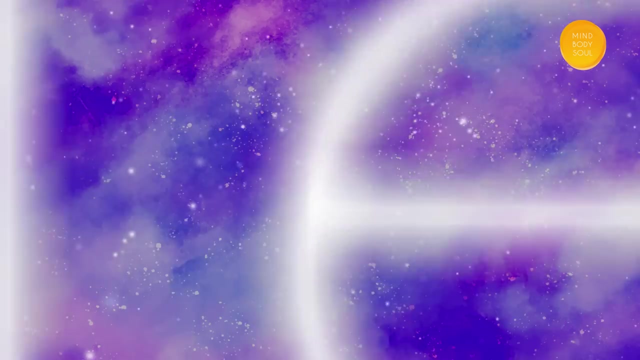 I let go of worries that drain my energy. I let go of worries that drain my energy. I let go of worries that drain my energy. I let go of people who impact me negatively. I let go of people who impact me negatively. I let go of all the negative feelings about myself. 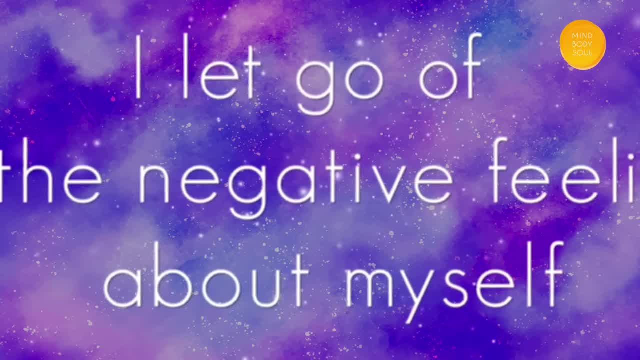 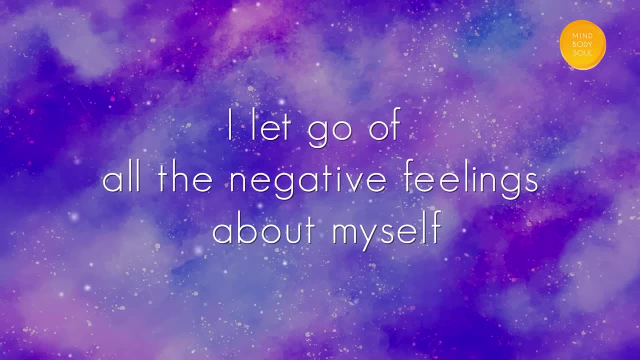 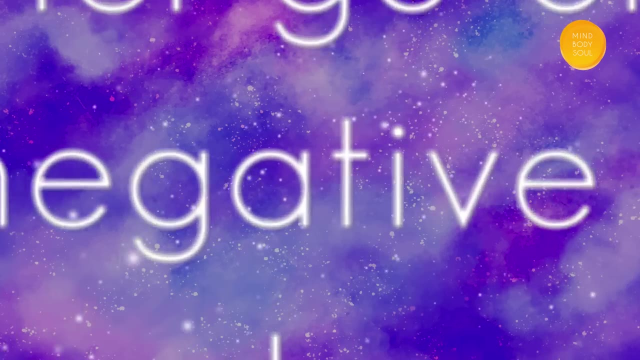 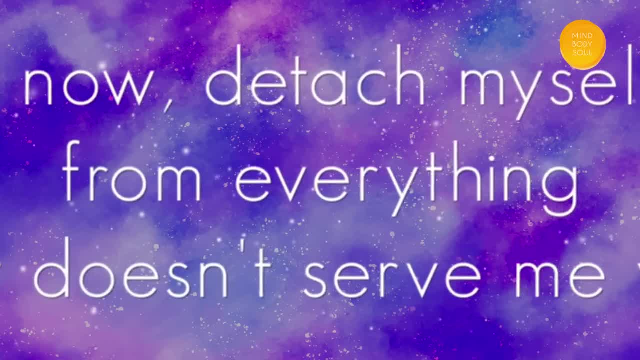 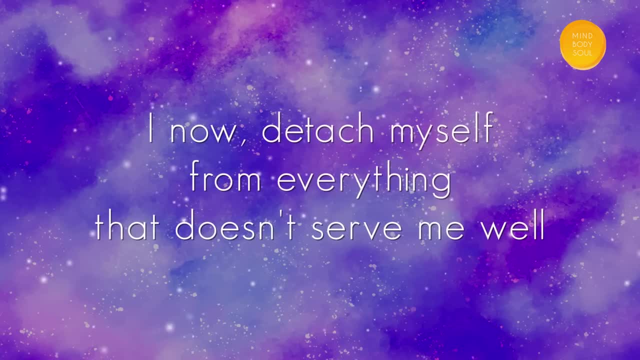 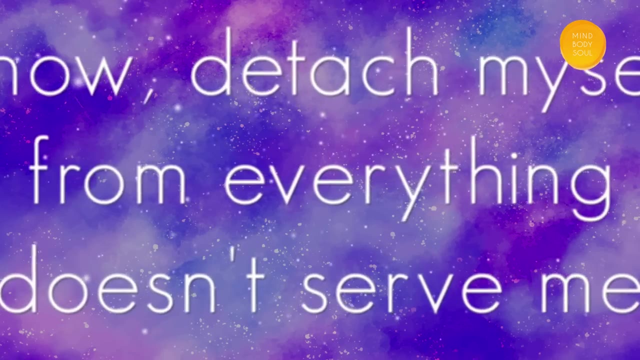 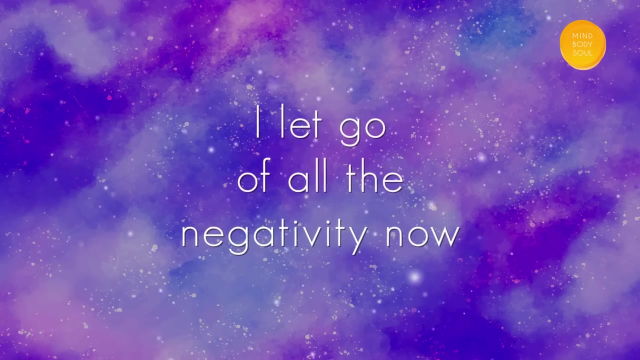 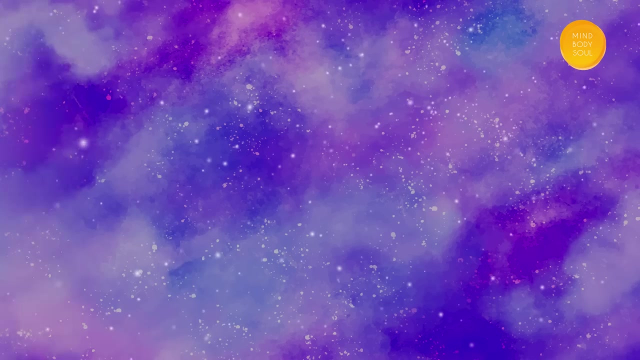 I now detach myself from everything that doesn't serve me well. I now detach myself from everything that doesn't serve me well. I now detach myself from everything that doesn't serve me well. I let go of all the negativity now. I let go of all the negativity now. 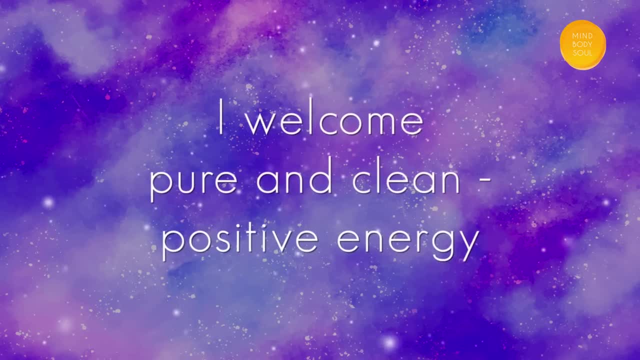 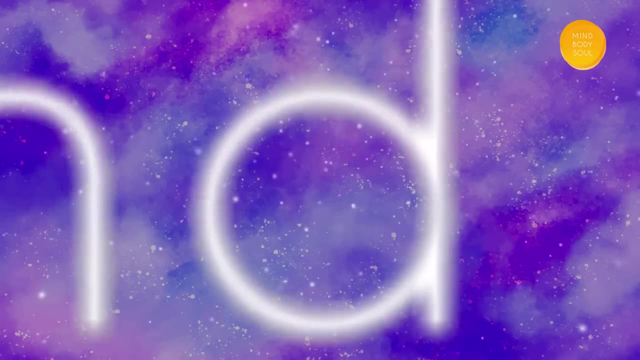 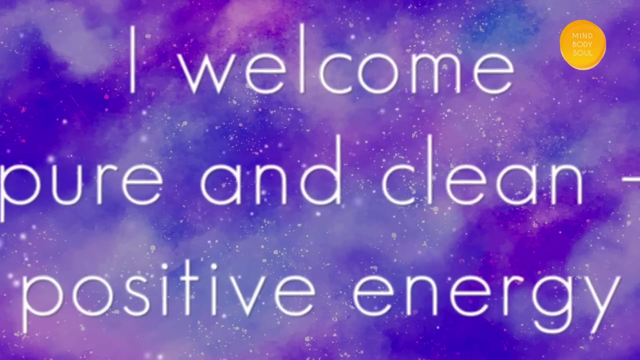 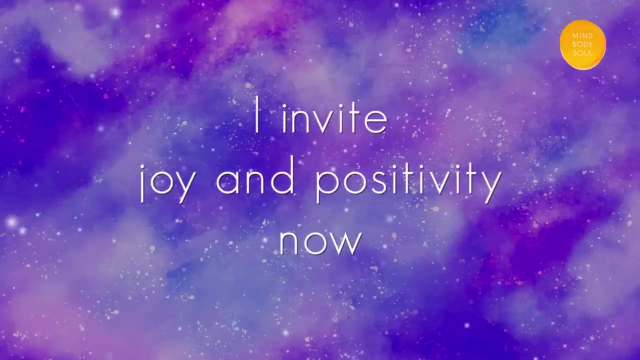 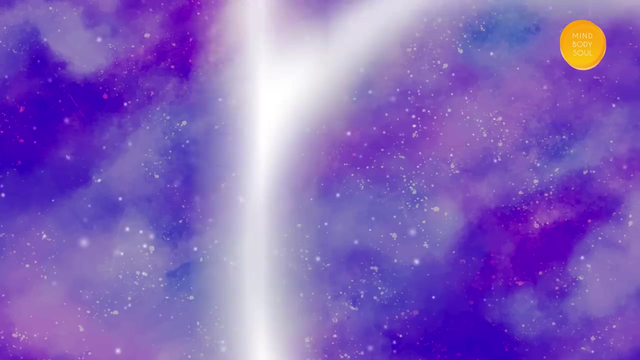 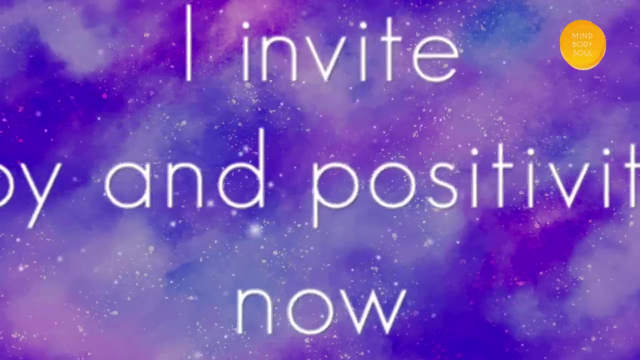 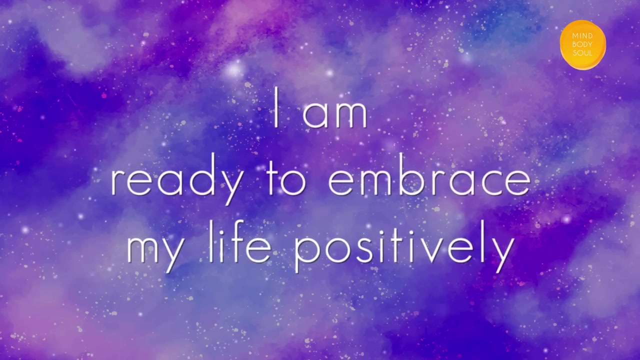 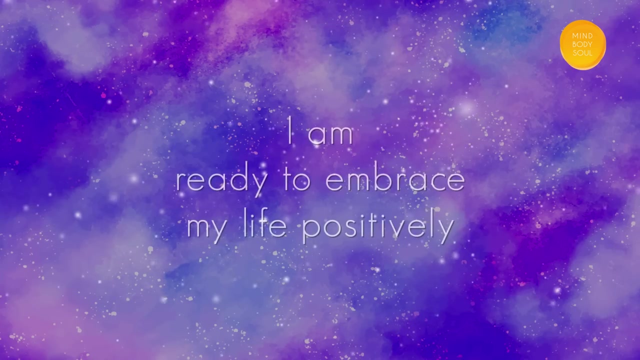 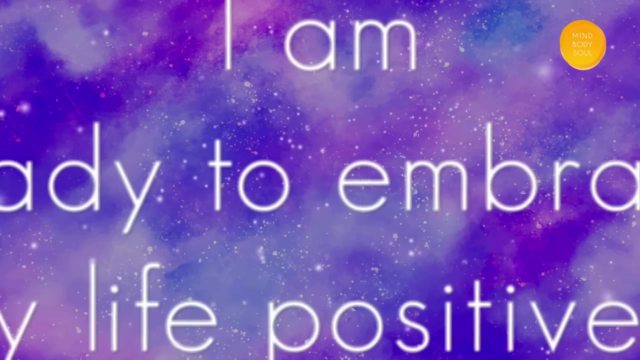 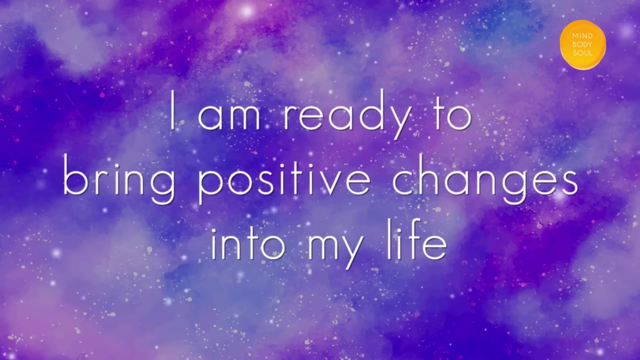 I welcome pure and clean positive energy. I welcome pure and clean positive energy. I invite joy and positivity now. I invite joy and positivity now. I am ready to embrace my life positively. I am ready to embrace my life positively. I am ready to bring positive changes into my life. 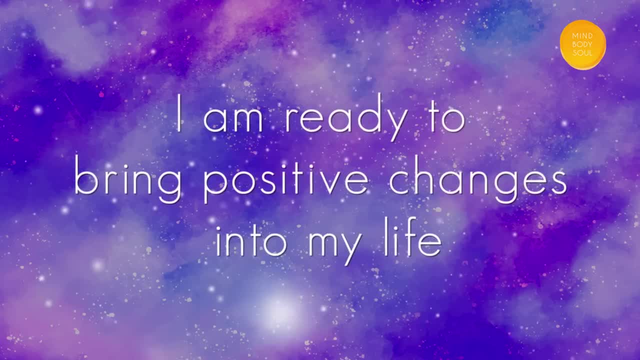 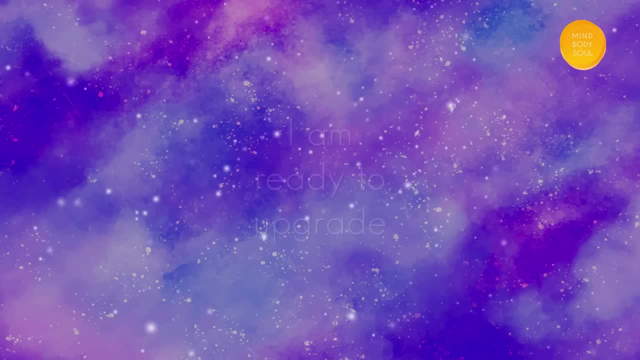 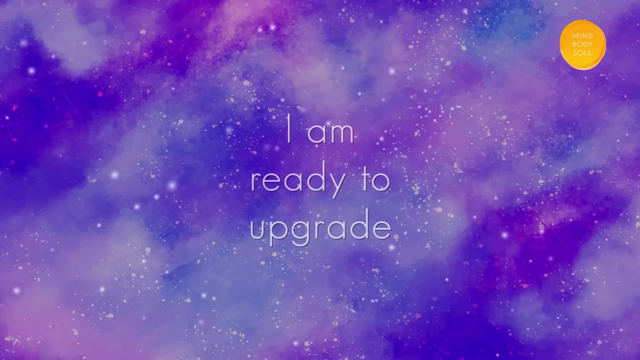 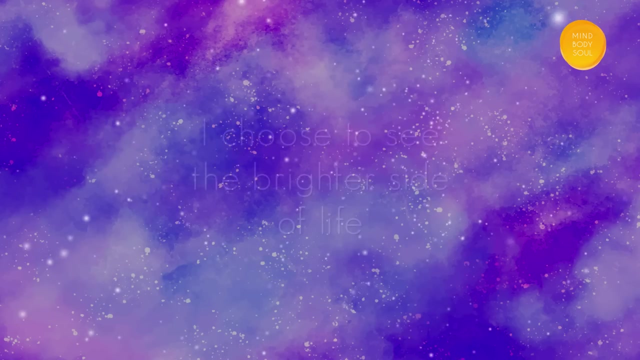 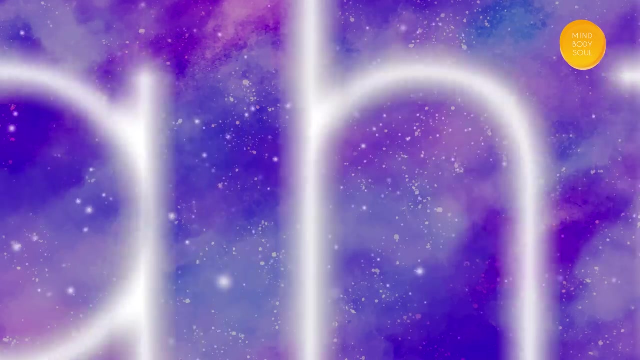 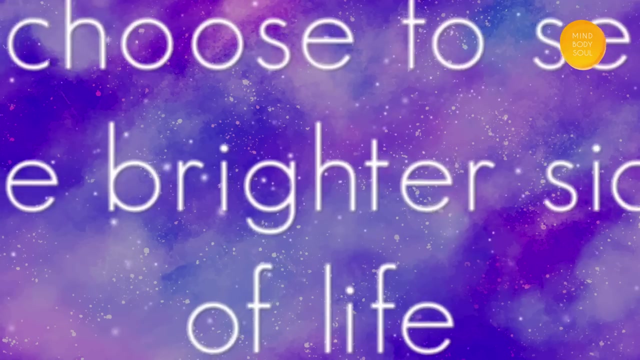 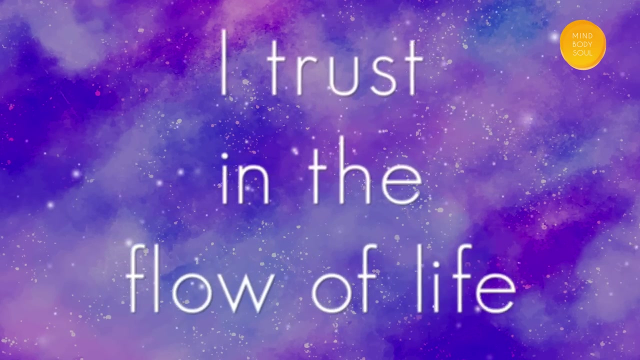 I am ready to bring positive changes into my life. I am ready to upgrade. I am ready to upgrade. I choose to see the brighter side of life. I choose to see the brighter side of life. I trust in the flow of life. 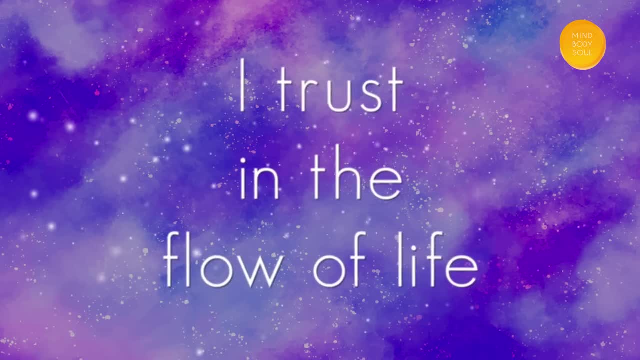 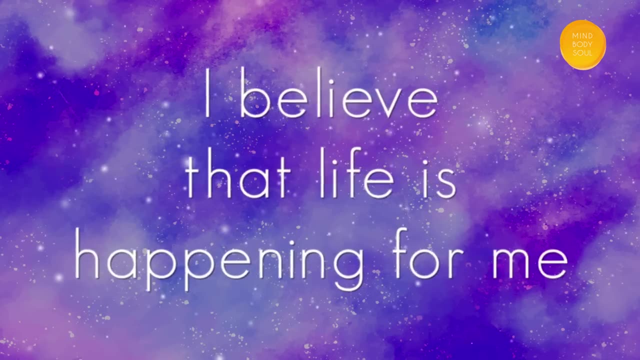 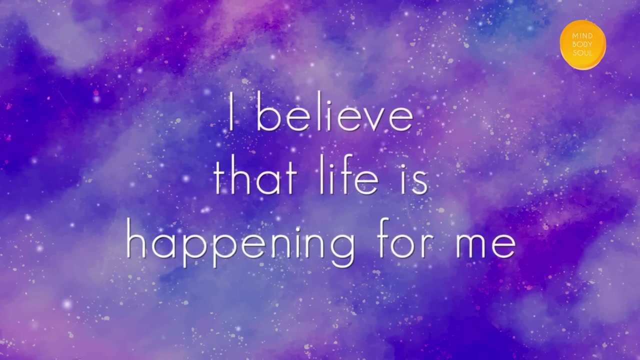 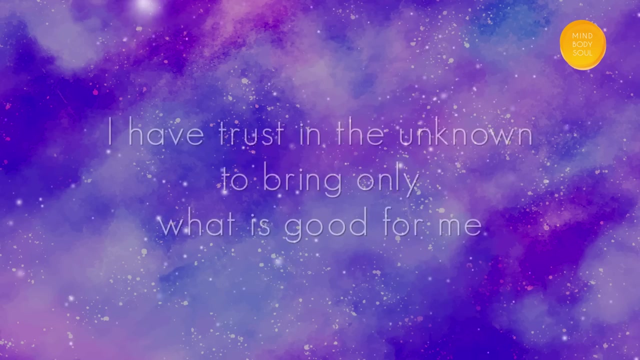 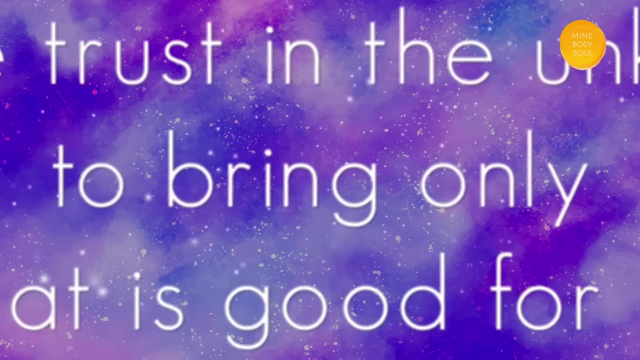 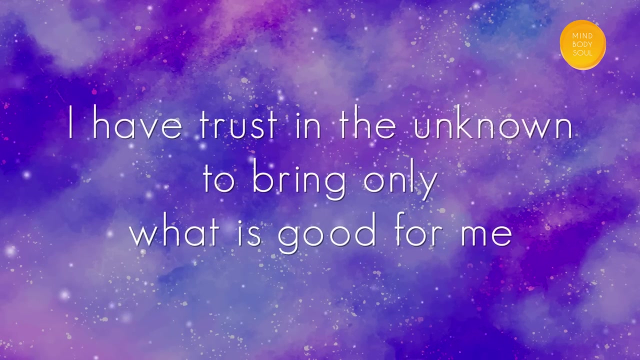 I trust in the flow of life. I believe that life is happening for me. I believe that life is happening for me. I have trust in the unknown to bring only what is good for me. I have trust in the unknown to bring only what is good for me. 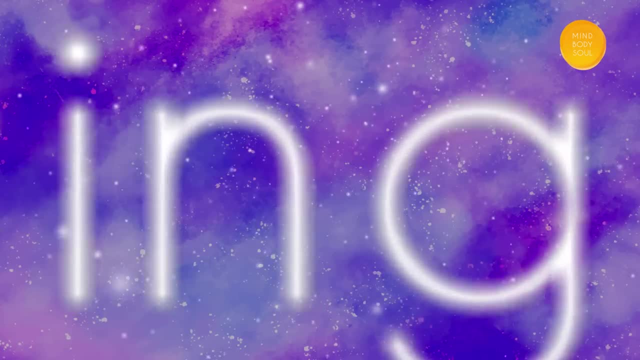 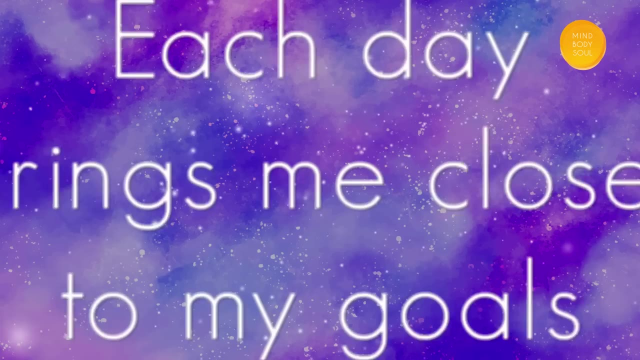 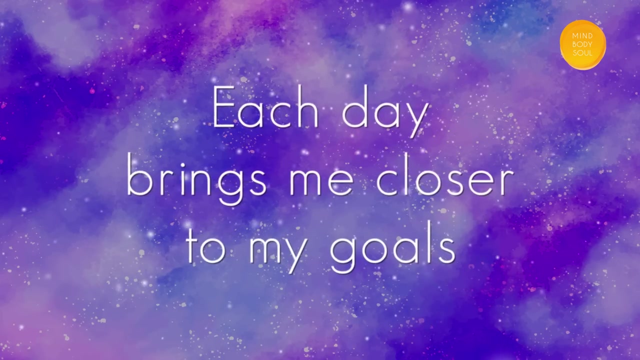 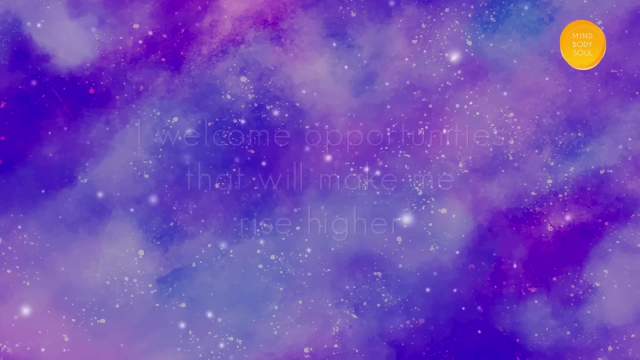 I have trust in the unknown to bring only what is good for me. Each day brings me closer to my goals. Each day brings me closer to my goals. I welcome opportunities that will make me rise higher. I welcome opportunities that will make me rise higher. 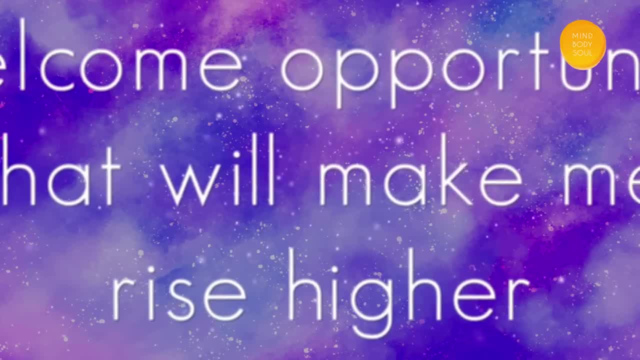 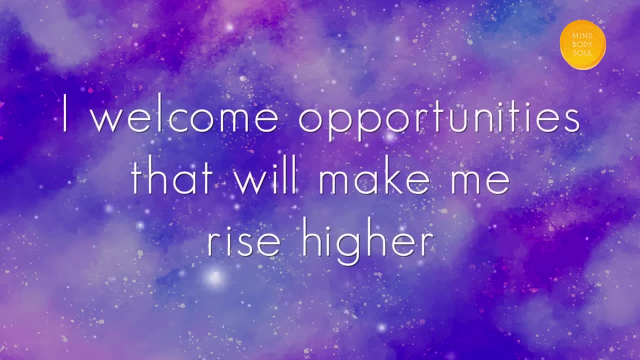 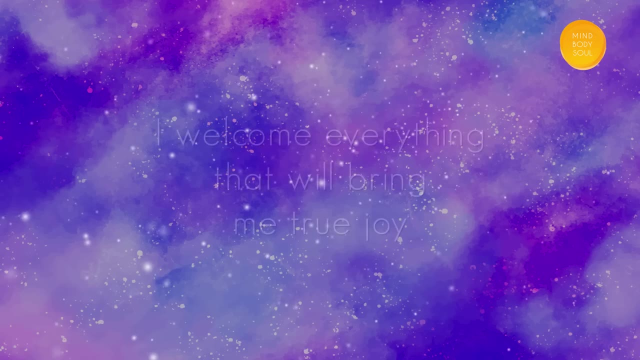 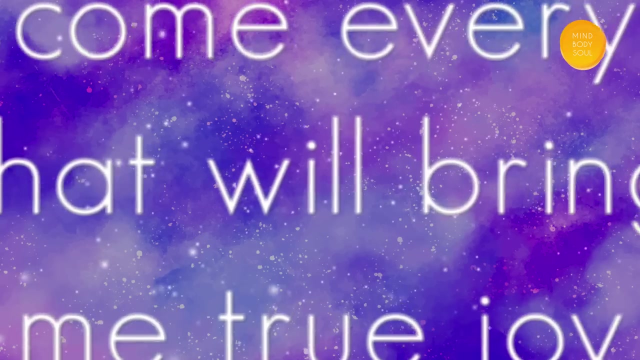 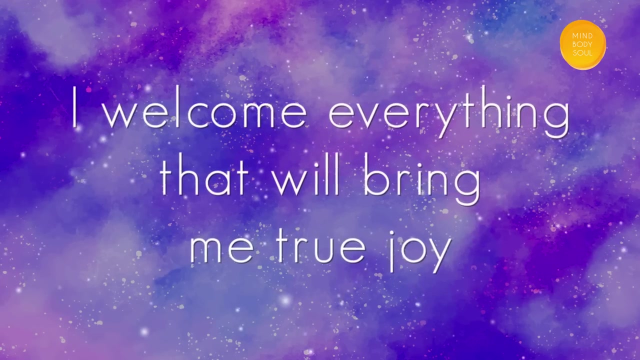 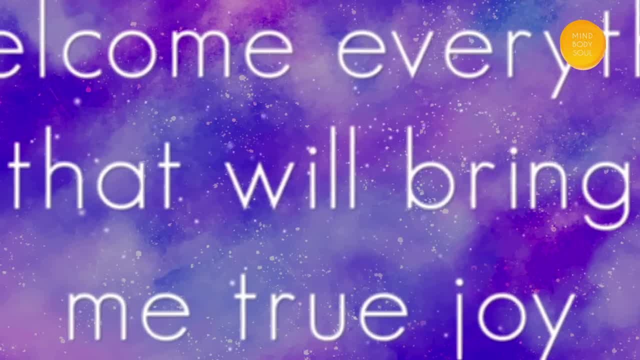 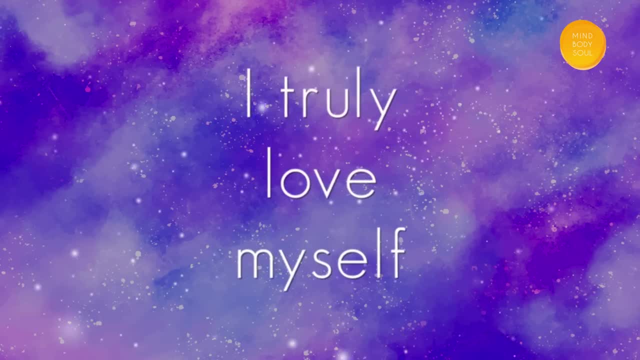 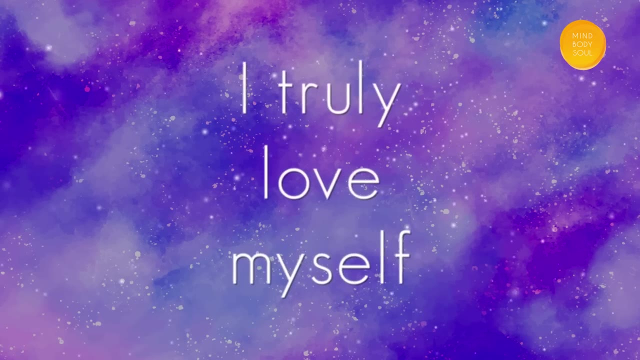 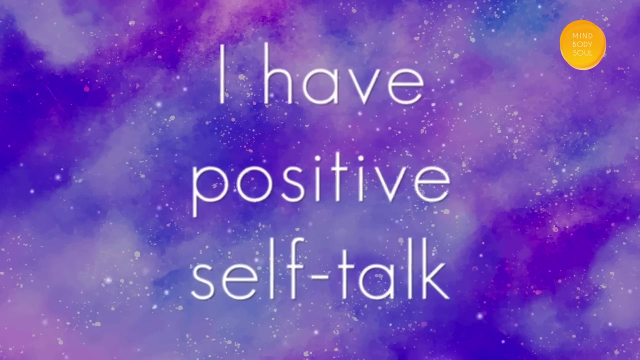 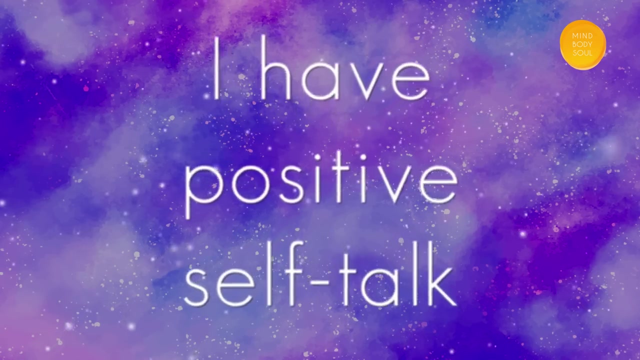 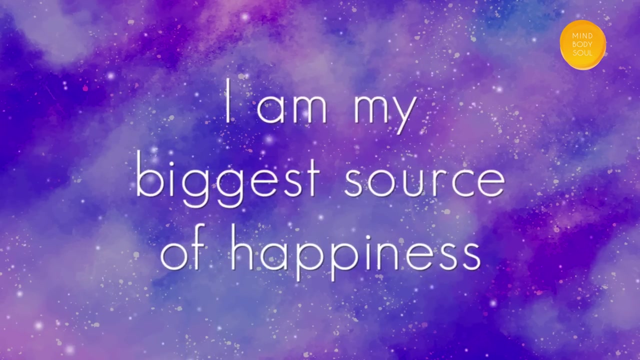 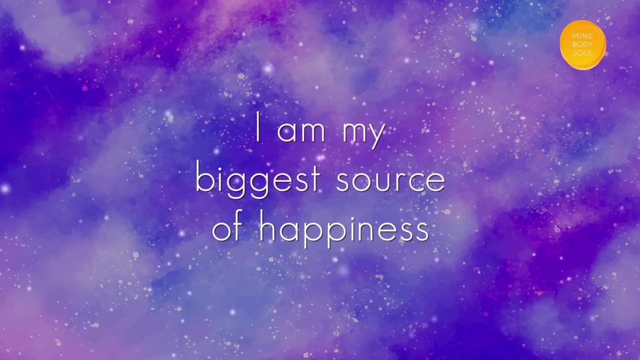 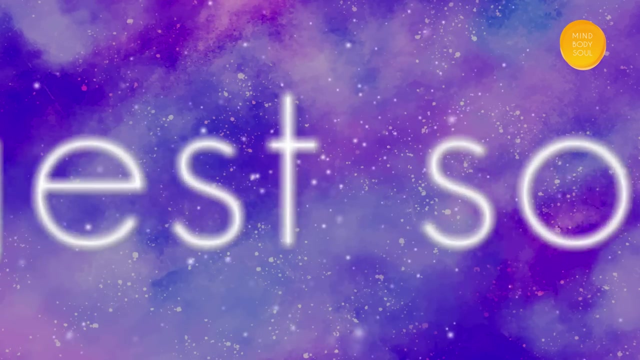 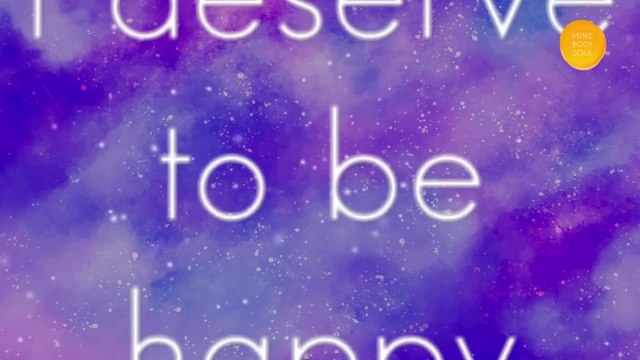 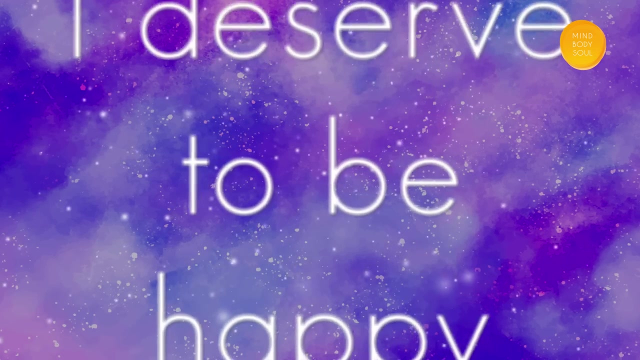 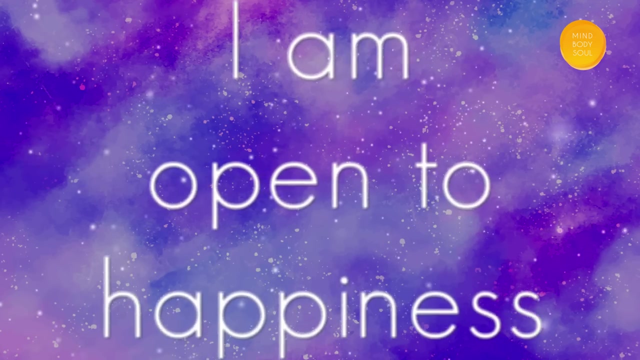 I truly love myself. I truly love myself. I have positive self-talk. I have positive self-talk. I am my biggest source of happiness. I am my biggest source of happiness. I deserve to be happy. I deserve to be happy. I am open to happiness. I am open to happiness. I am open to happiness. I am open. 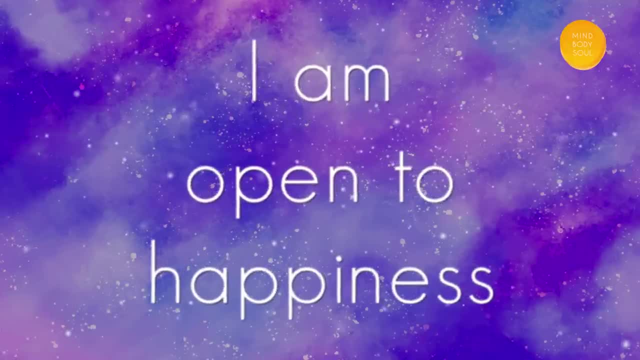 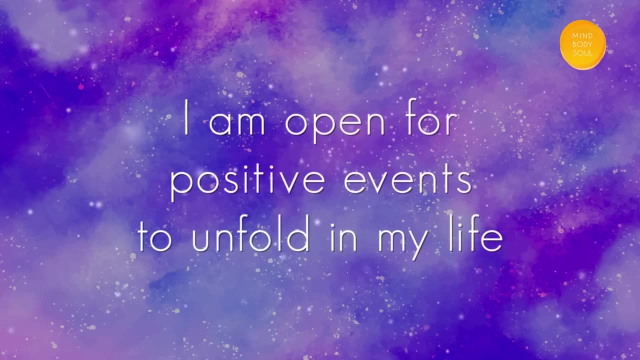 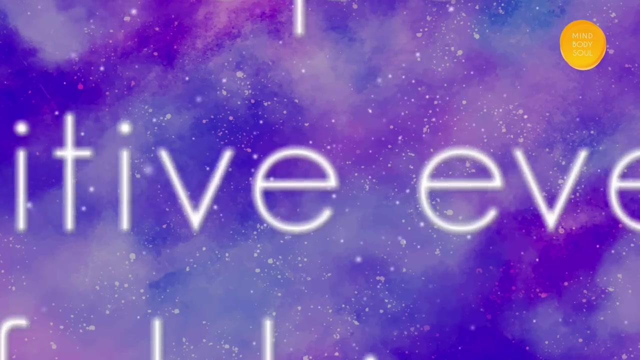 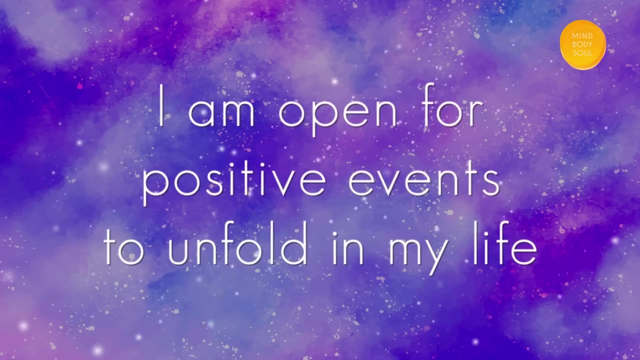 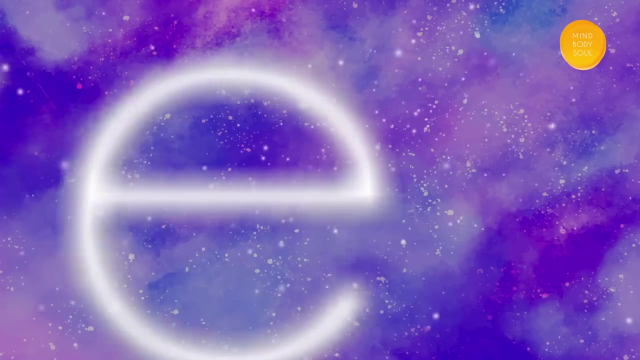 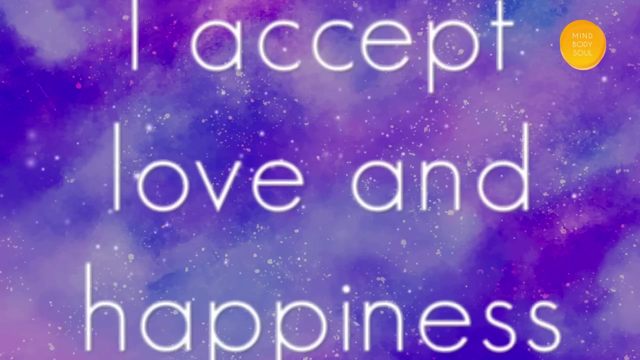 I am open to happiness. I am open for positive events to unfold in my life. I am open for positive events to unfold in my life. I am open for positive events to unfold in my life. I accept love and happiness. I accept love and happiness. 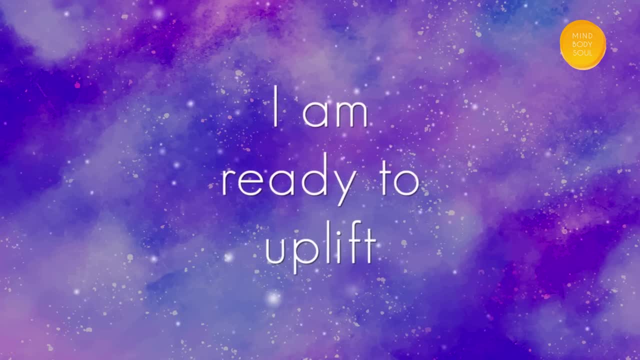 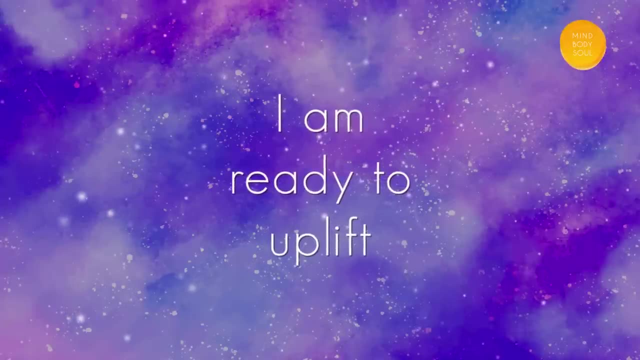 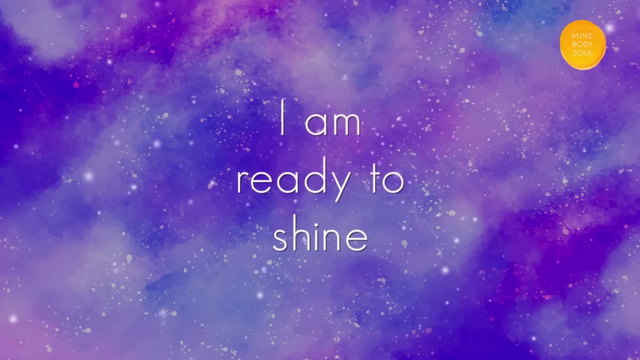 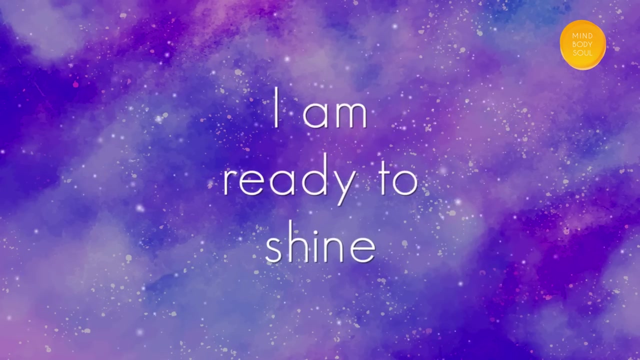 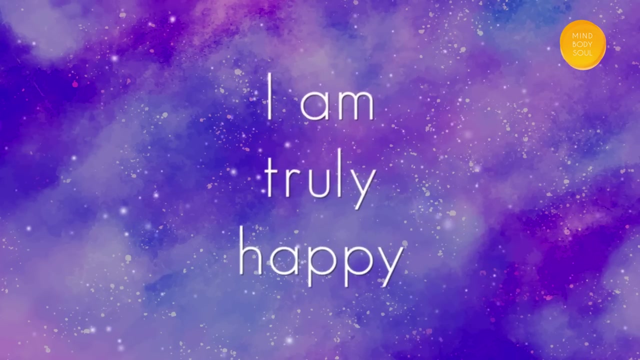 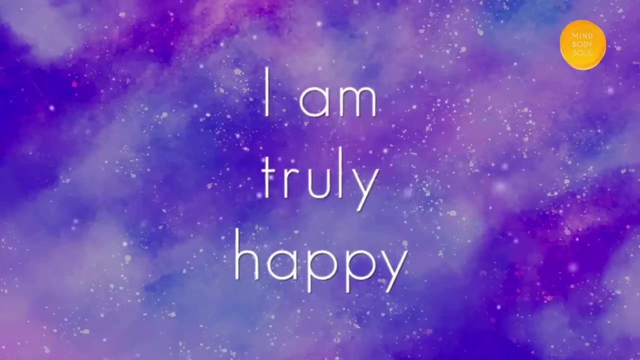 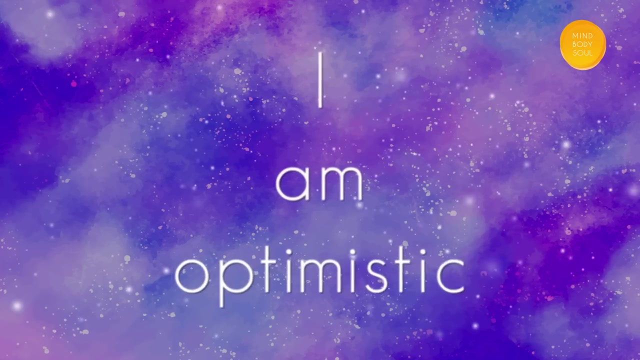 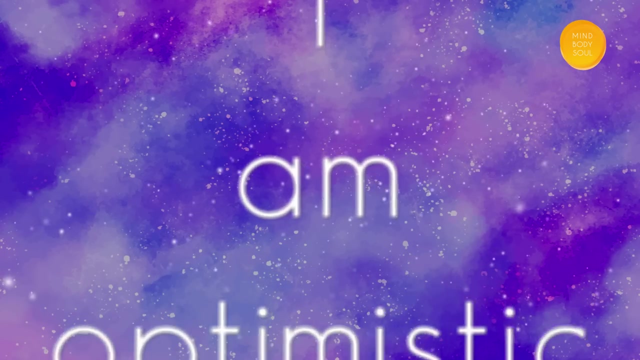 I am ready to uplift. I am ready to uplift. I am ready to uplift. I am ready to shine. I am ready to shine. I am truly happy. I am truly happy. I am optimistic, I am optimistic, I am hopeful. 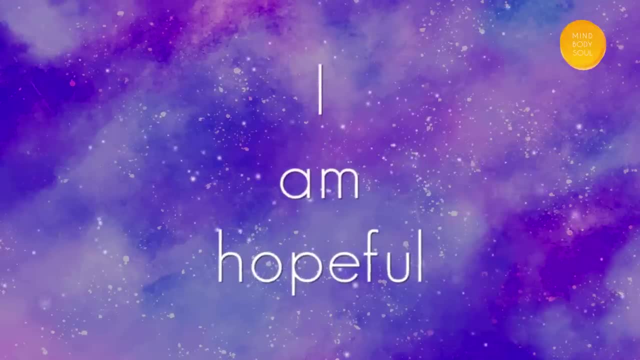 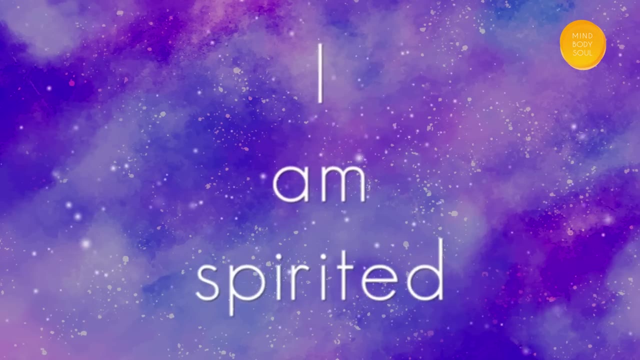 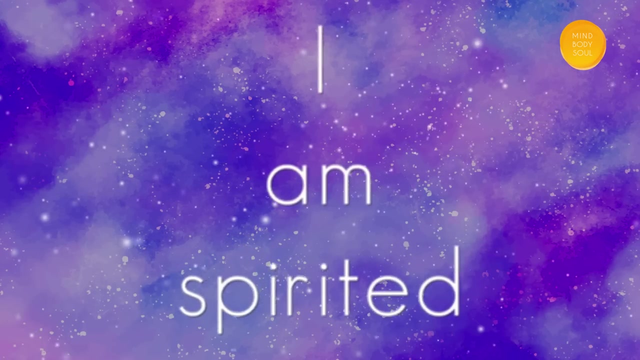 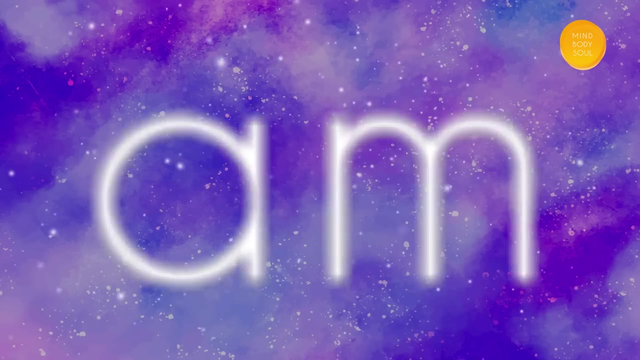 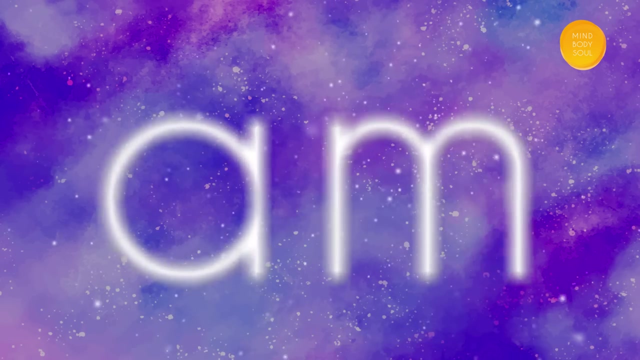 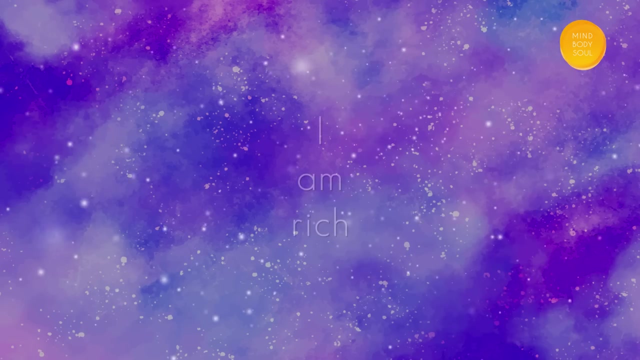 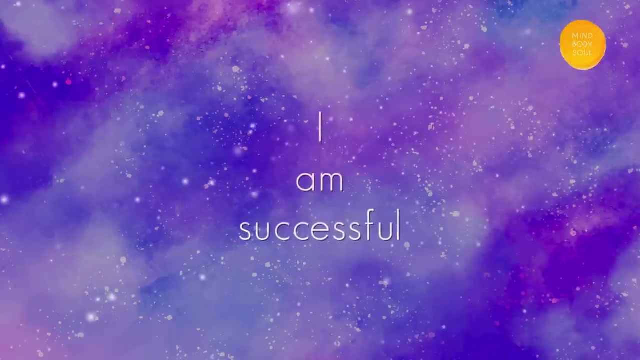 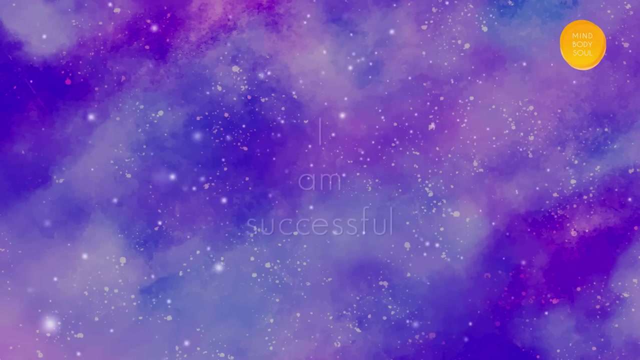 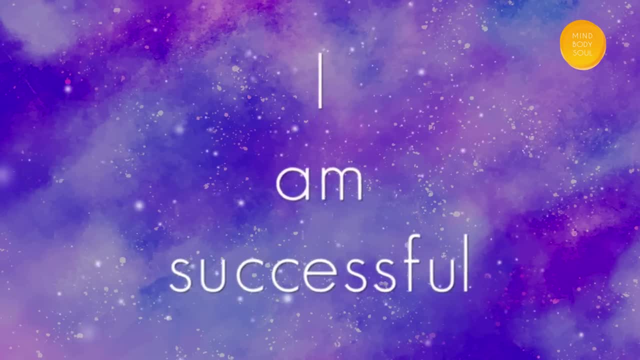 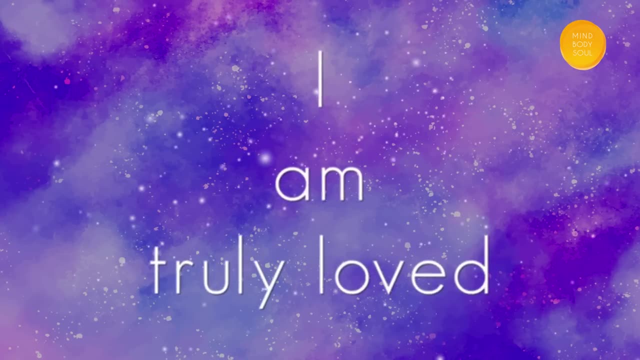 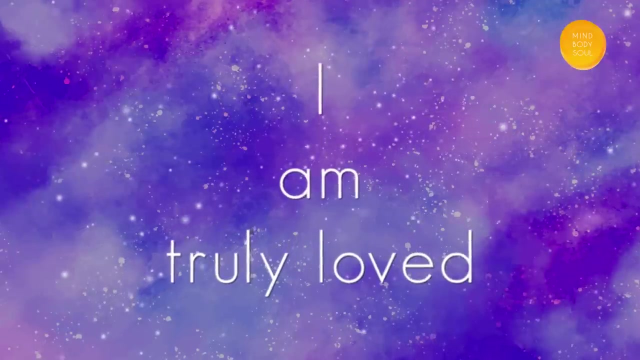 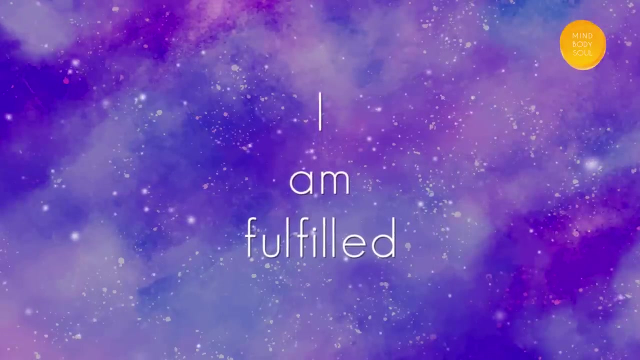 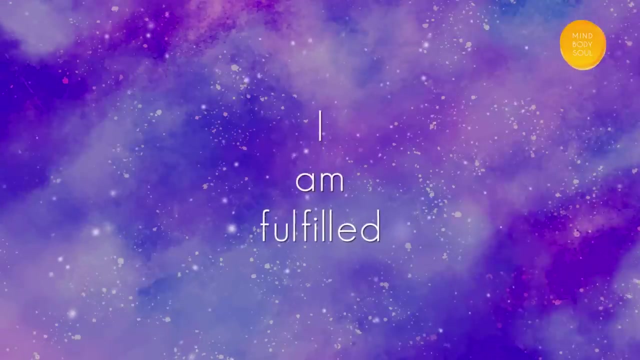 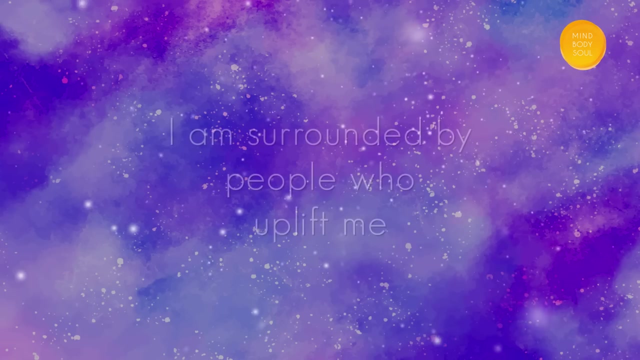 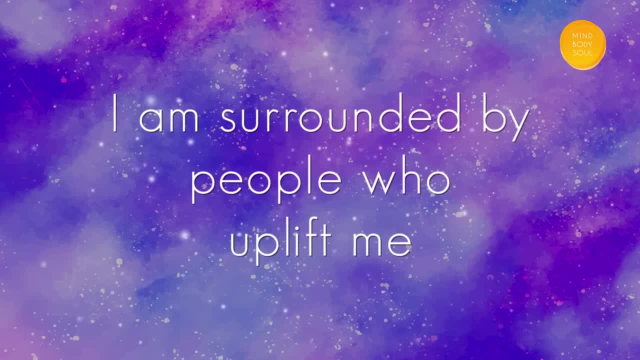 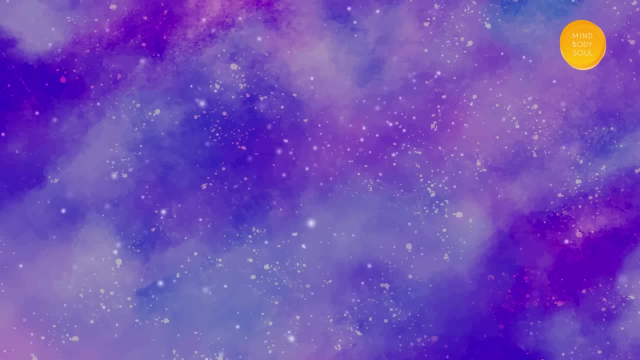 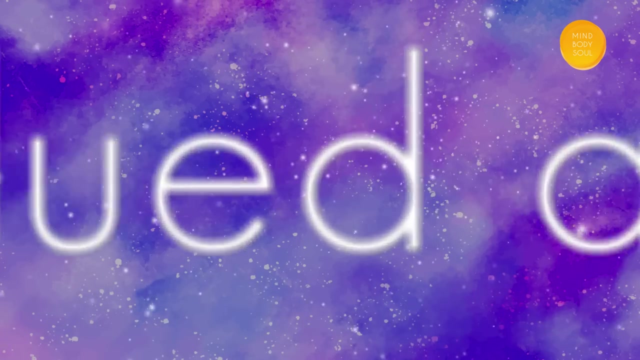 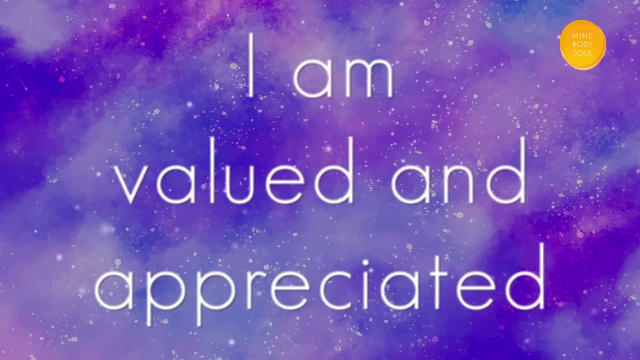 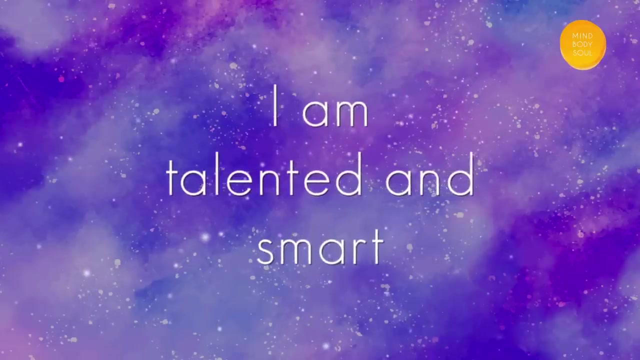 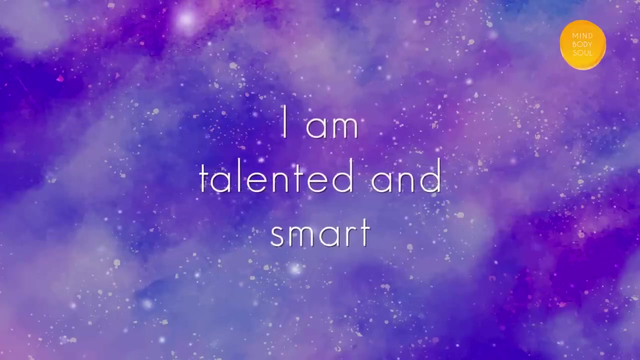 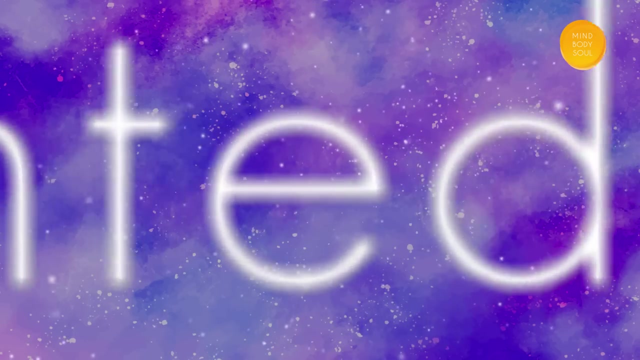 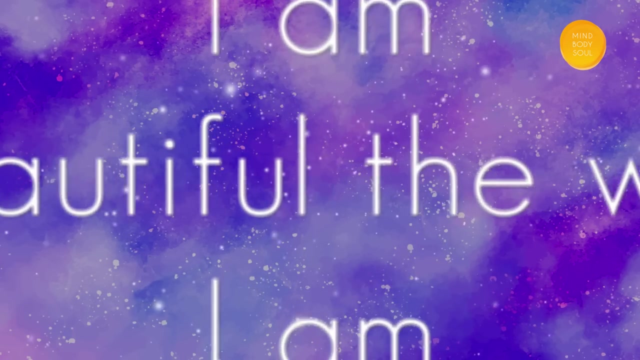 I am surrounded by people who uplift me. I am valued and appreciated. I am valued and appreciated. I am talented. I am talented and smart. I am talented and smart. I am beautiful the way I am. I am beautiful the way I am. 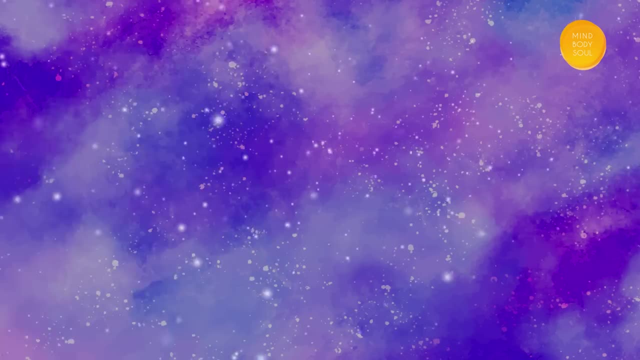 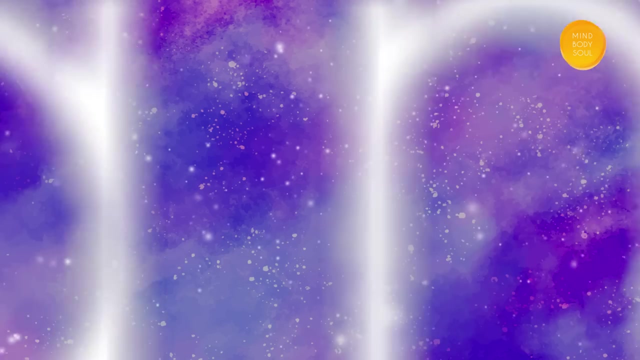 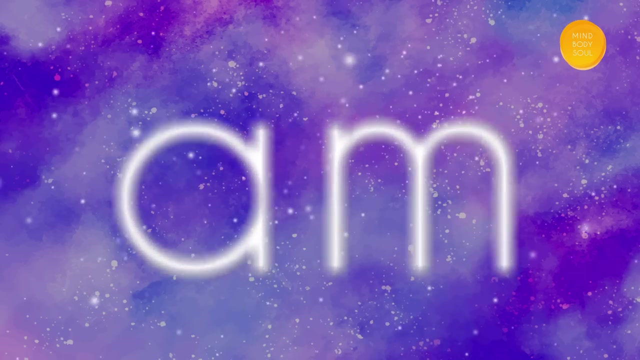 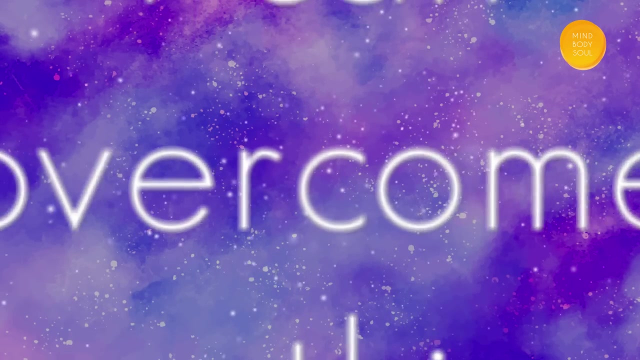 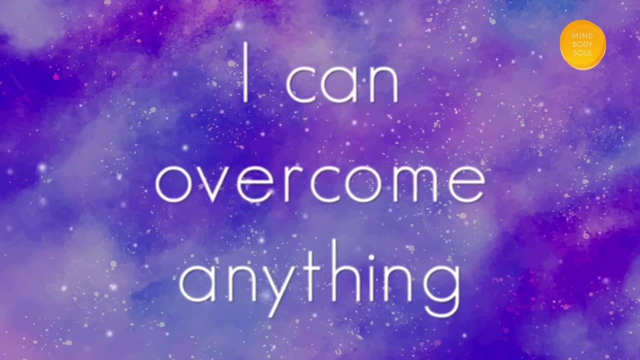 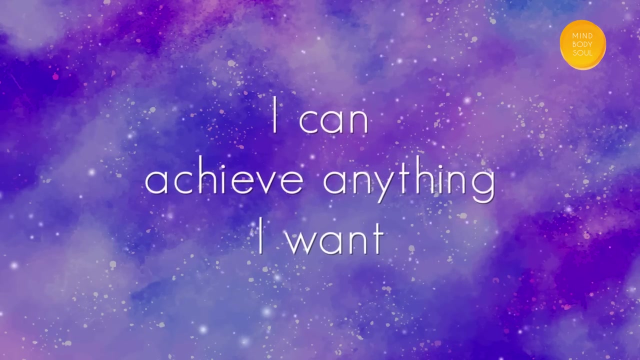 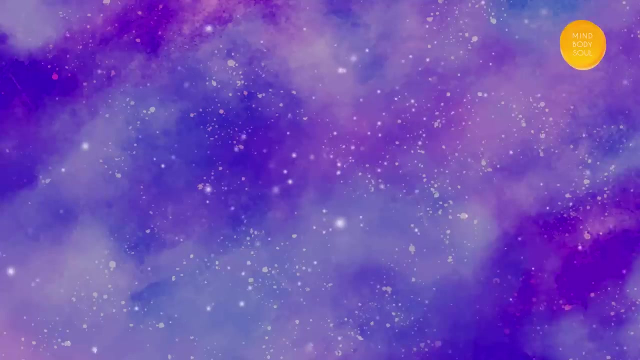 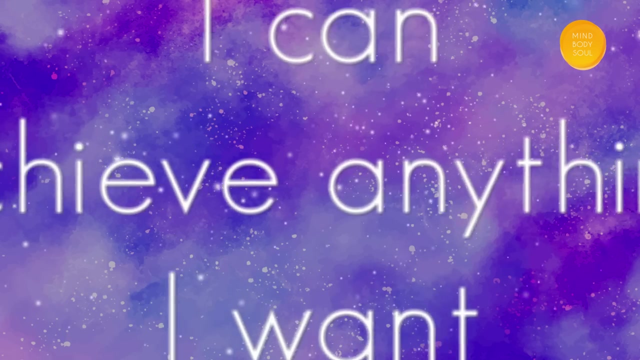 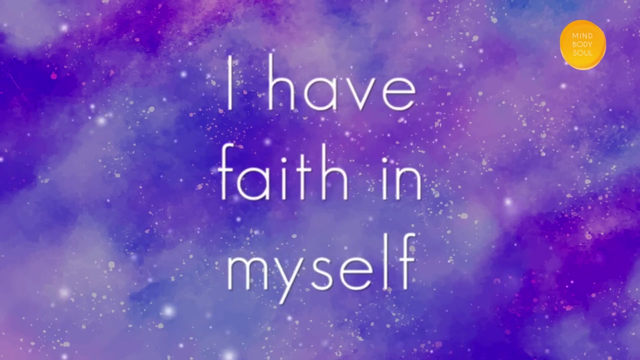 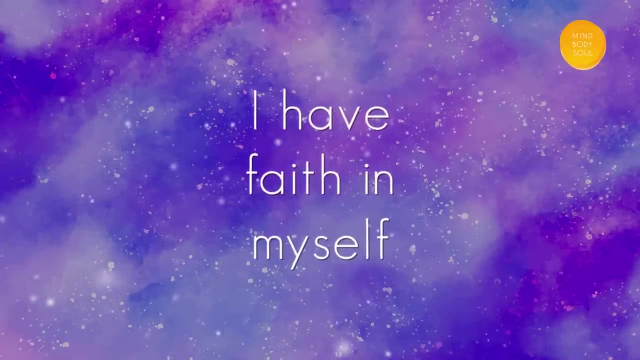 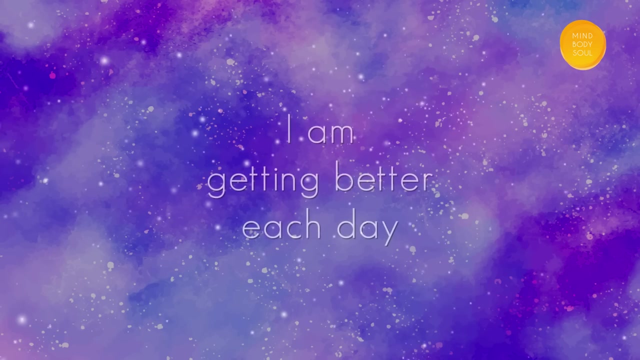 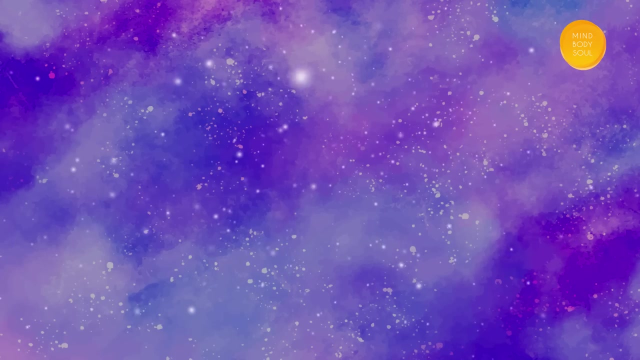 I am strong. I am strong, I can overcome anything. I can overcome anything. I can achieve anything I want. I can achieve anything I want. I have faith in myself. I have faith in myself. I am getting better each day. I am getting. 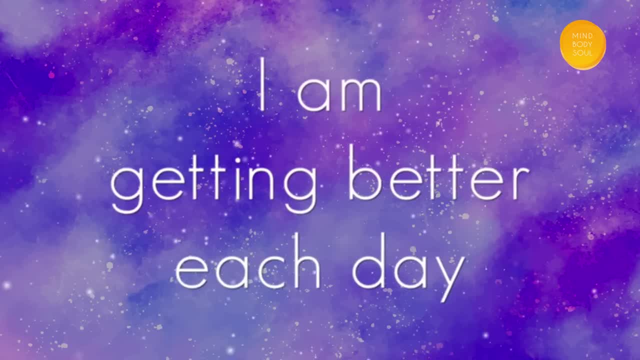 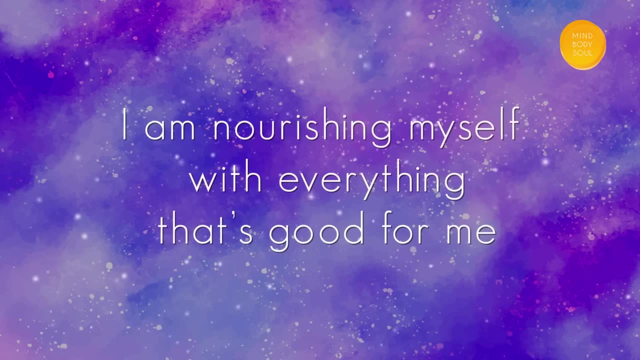 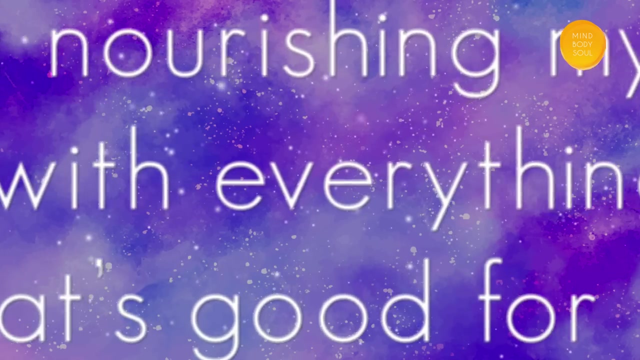 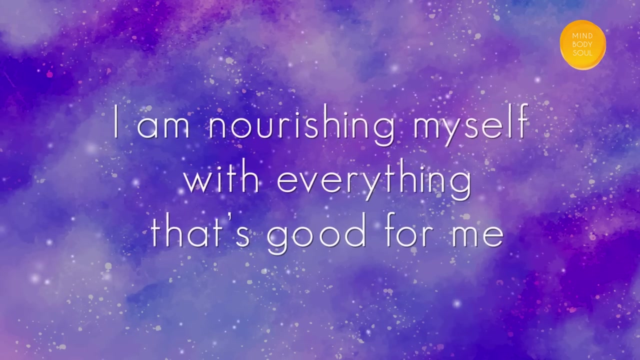 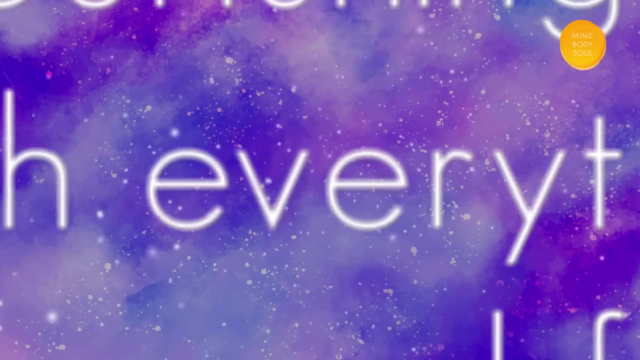 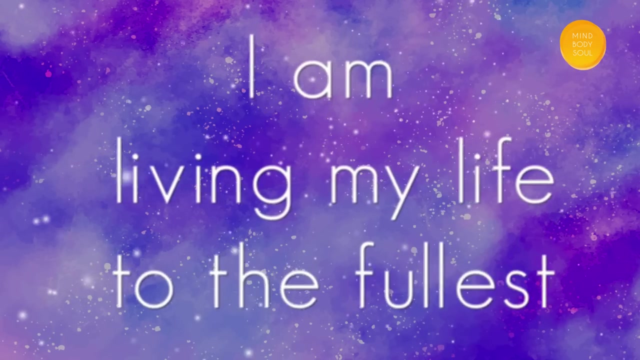 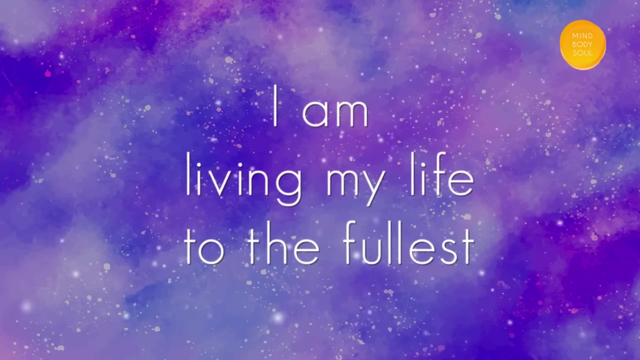 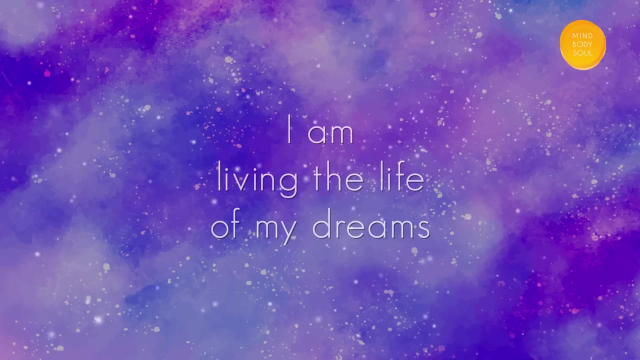 better each day. I am nourishing myself with everything that's good for me. I am nourishing myself with everything that is good for me. I am living my life to the fullest. I am living my life to the fullest. I am living the life of my dreams. 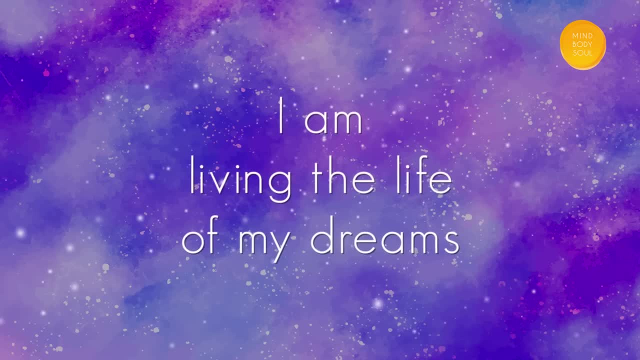 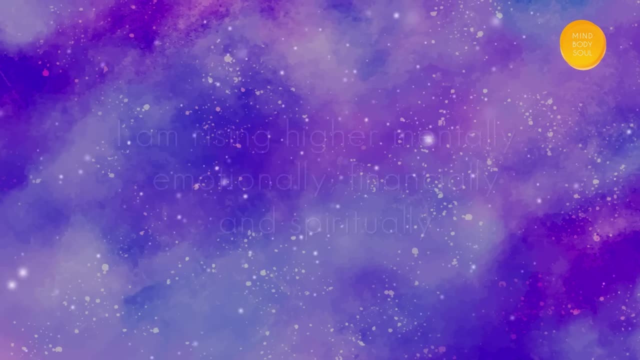 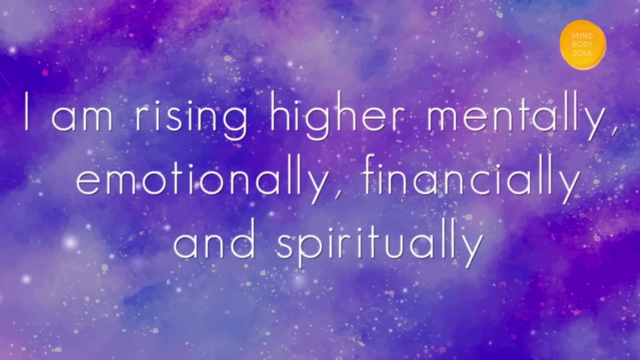 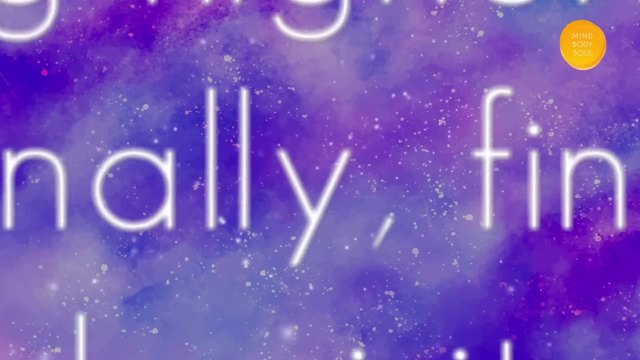 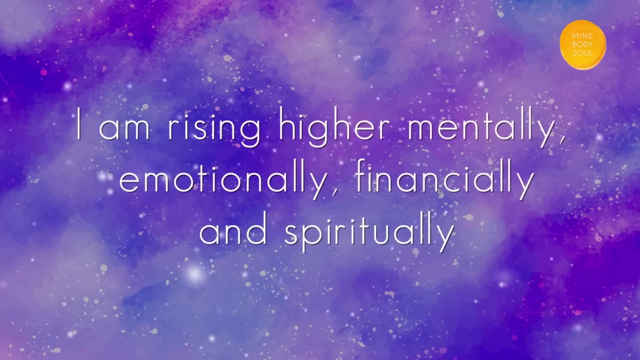 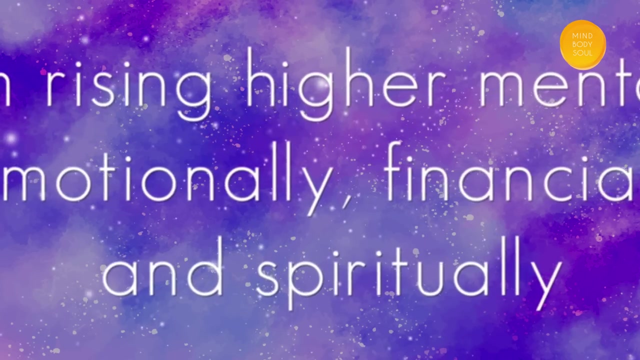 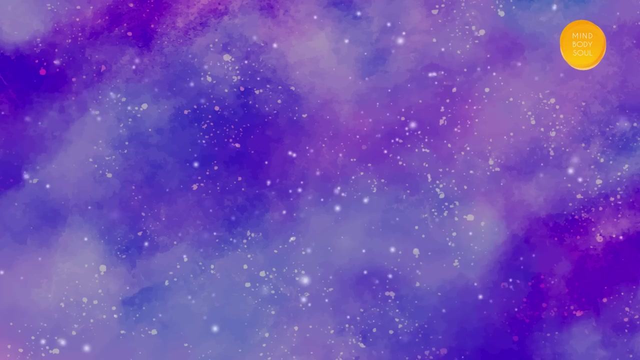 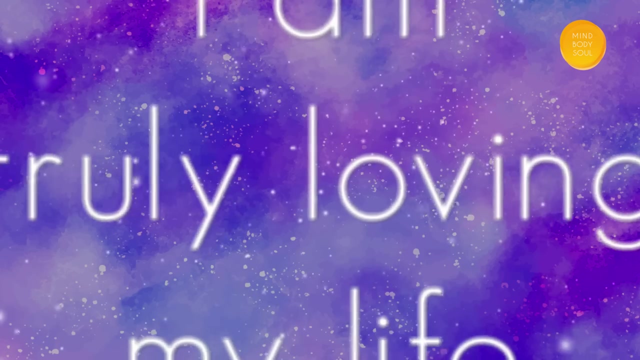 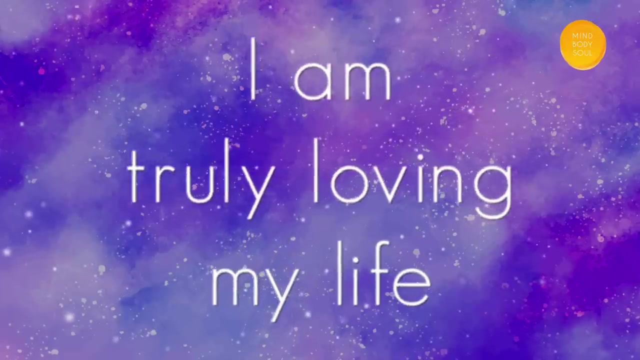 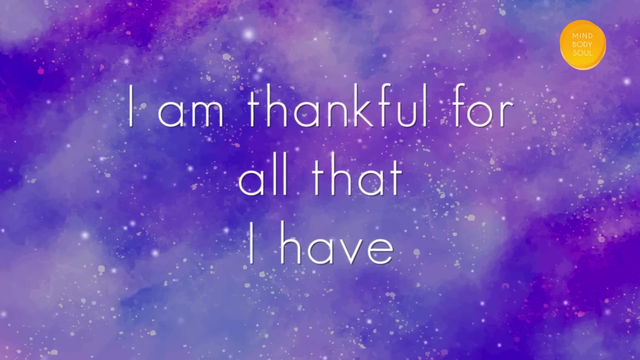 I am living the life of my dreams. I am rising higher mentally, emotionally, financially and spiritually. I am rising higher mentally, emotionally, financially and spiritually. I am truly loving my life. I am truly loving my life. I am thankful for all that I have. 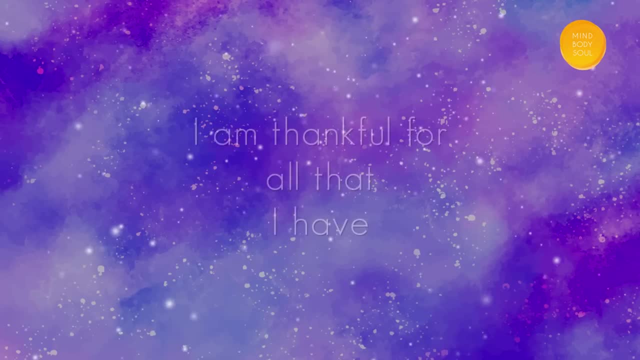 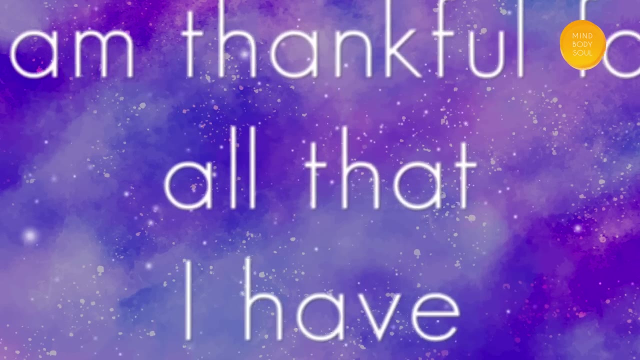 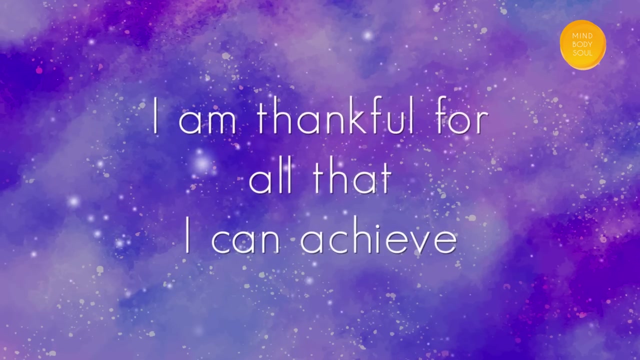 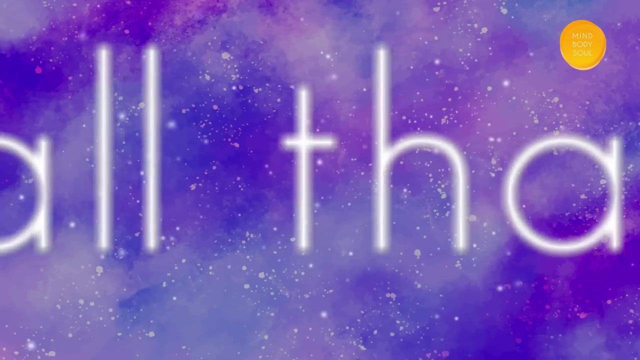